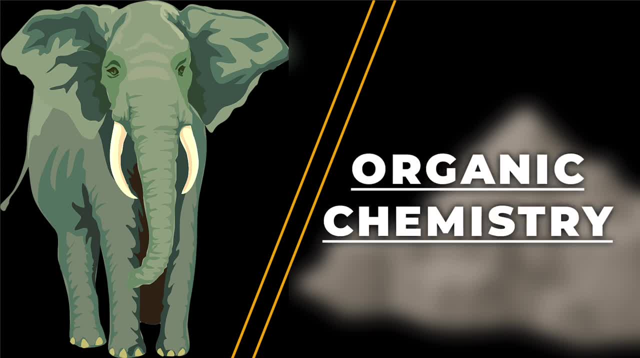 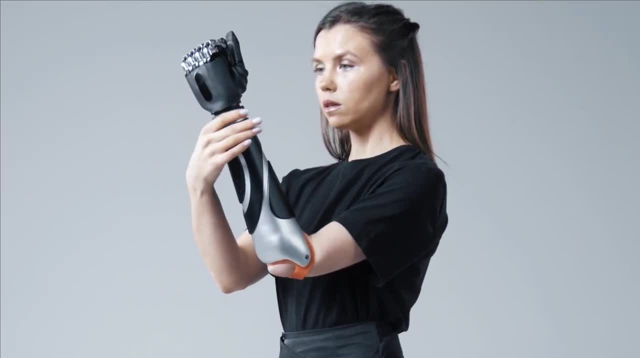 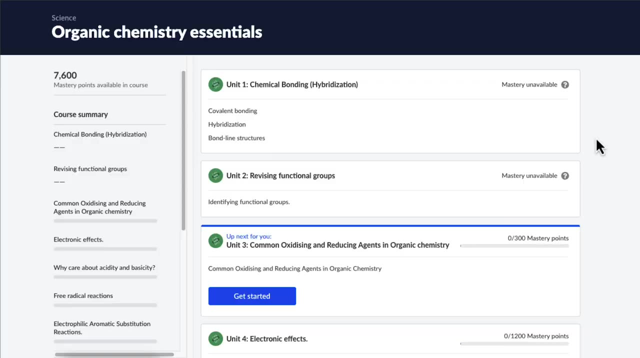 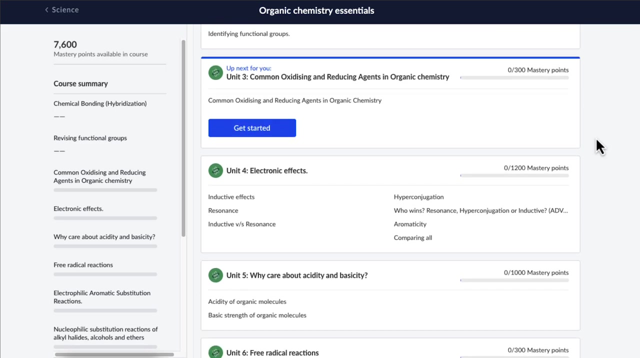 eventually life itself. Welcome to organic chemistry. It's the branch of chemistry that helps us create new medicines, develop innovative materials and unlock the secrets of life itself. If you're excited, let's dive right in. Although this course is aligned with CBSE class 11th and 12th curriculum, you can see it's sequenced quite differently. 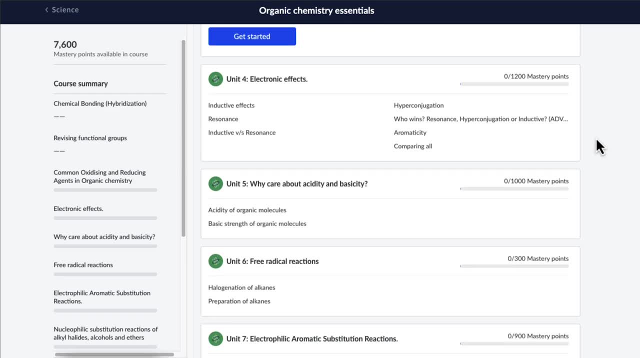 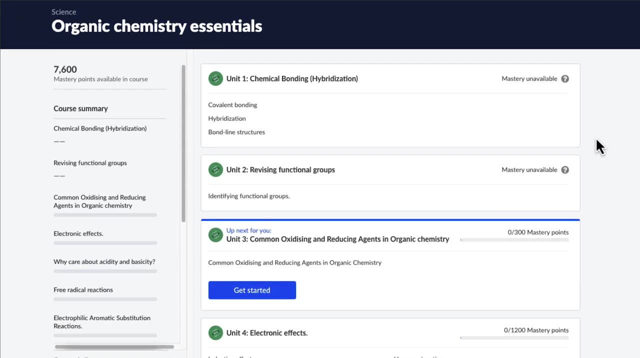 from your textbooks, And that's because we think this way, you will learn about the reactions and mechanisms very logically, Something I always wanted to do. That's why, after first learning the basics of life, we're going to talk about how to create new medicines. 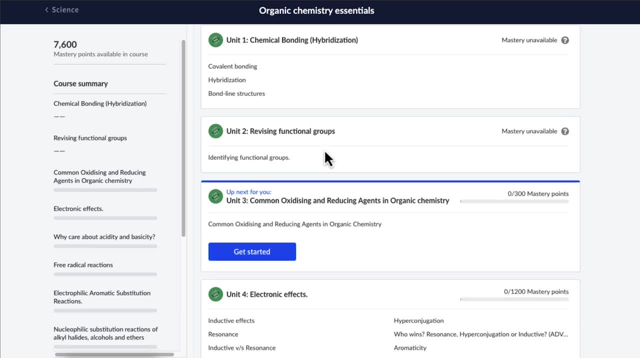 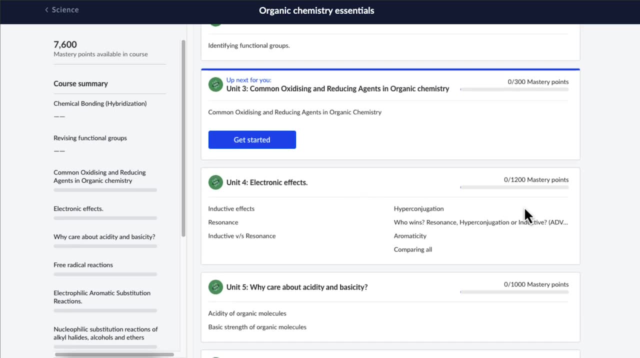 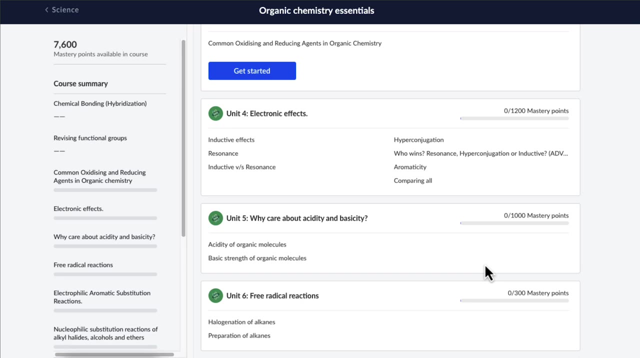 and develop innovative materials and unlock the secrets of life itself. If you're excited, the basics like chemical bonding, functional groups and some other reactions. we will first understand all the electronic effects that are at play over here. We'll then use that to understand about acidity and basicity And then we will use all that to learn different. 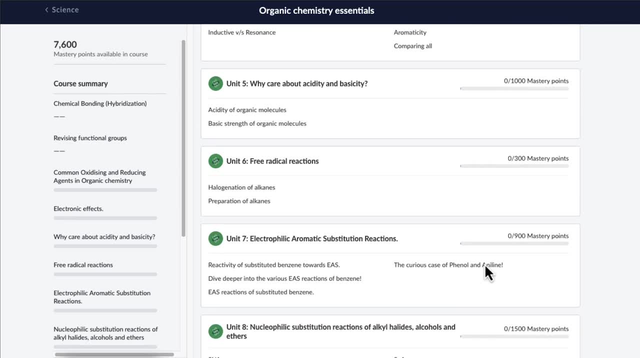 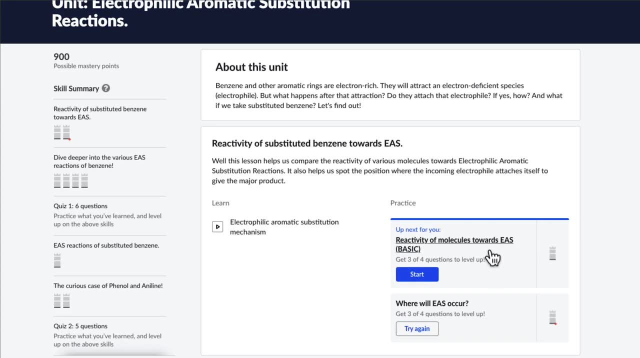 kinds of reactions like addition, substitution, elimination and whatnot, And inside each unit you'll find videos to help you understand the basics of life itself, And then we'll talk about the basics of life itself, And then you have exercises where you can practice. 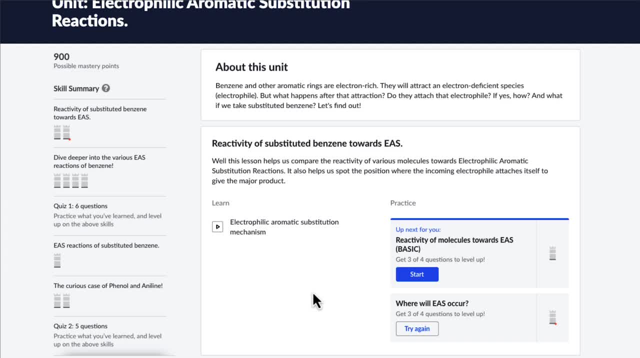 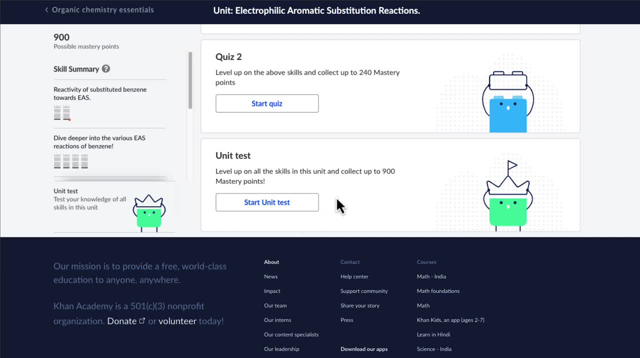 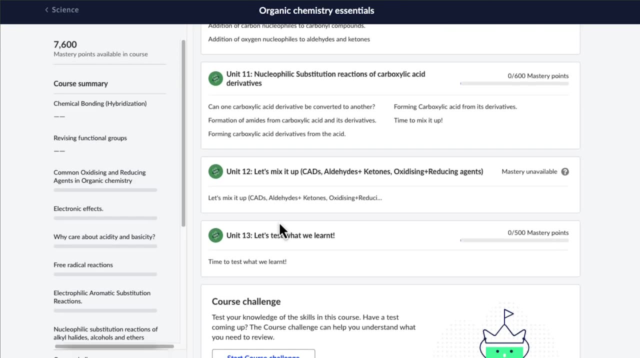 different kinds of questions related to that particular topic, And then you have quizzes and unit tests, which jumbles all the questions together, So you can totally gain mastery over this entire unit, And then, towards the end of the course, you'll be able to put everything. 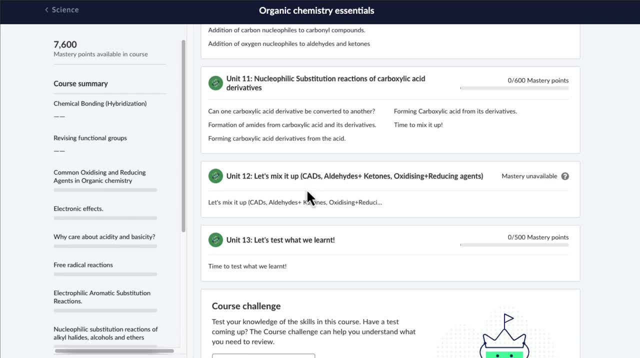 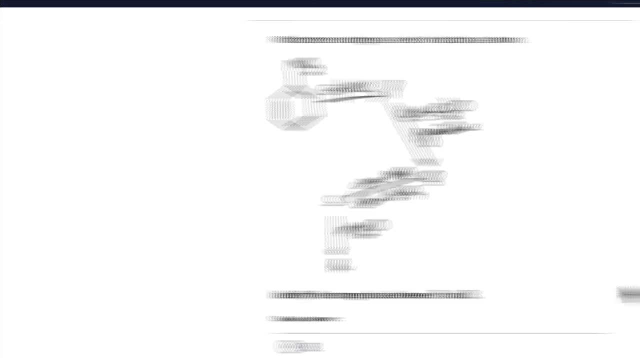 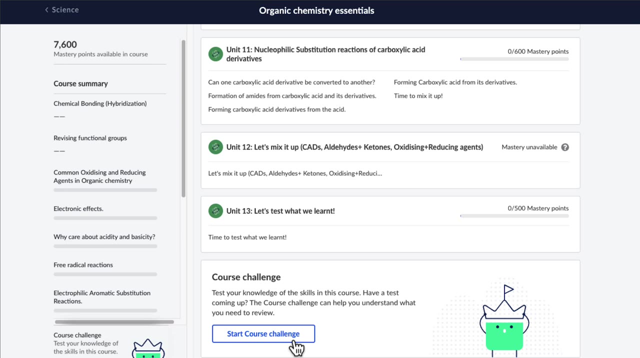 that you learned earlier, to logically predict how reactions would go, what products would be formed, compare stabilities, identify reagents and so much more. And finally, you can take a course challenge to test your understanding of this entire course, And so you can see.